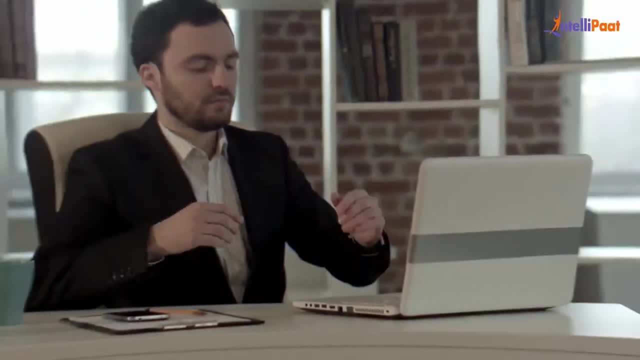 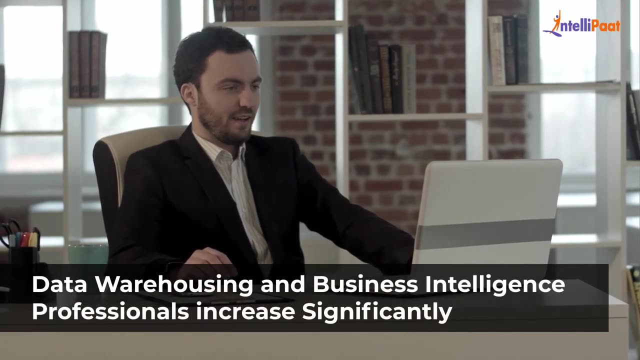 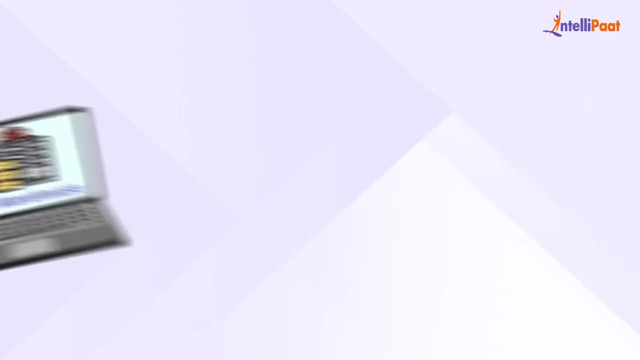 It is interesting to note that the salaries of data warehousing and business intelligence professionals increase significantly with each additional years of expertise. Now, before we discuss our today's agenda, do not forget to hit the subscribe button and click the bell icon. So first we will discuss about what is data warehouse architecture. 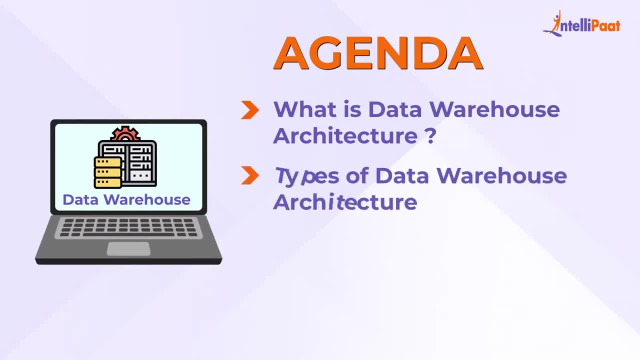 Moving ahead, we will discuss about types of data warehouse architecture. Then we will discuss about properties of data warehouse architecture. Moving ahead, we will discuss about single tier architecture. Then we will discuss about two tier architecture. Moving ahead, we will discuss about three tier architecture. 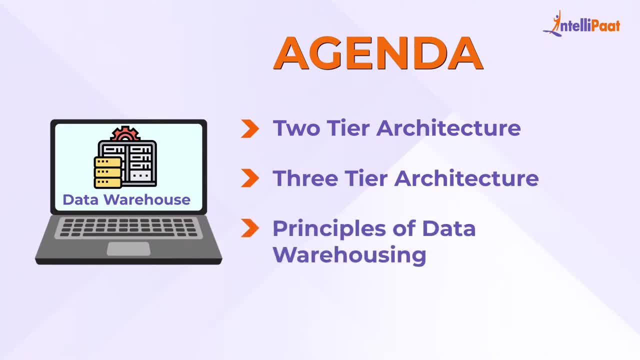 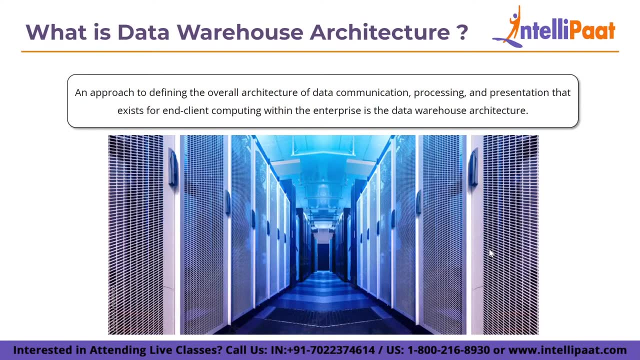 And at the end we will discuss about principles of data warehousing. So let's start with data warehouse architecture. Data warehouse architecture is an approach to define the overall architecture of data communication, processing and presentation. The first tier architecture that exists for end client computing within the enterprise is actually called the data warehouse architecture. 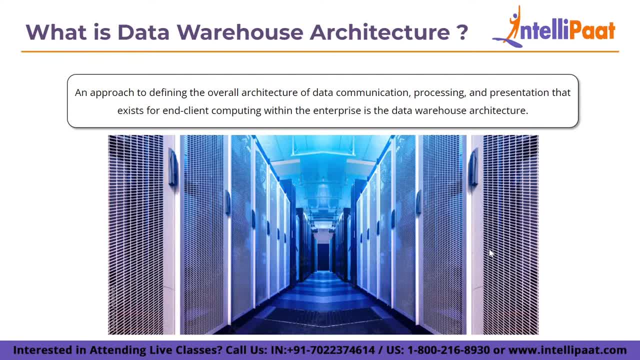 Although every data warehouse is unique, they all share certain essential elements. Online transaction processing is built into the production applications, like payroll accounts, payable, product purchasing and inventory control. These programs collect thorough information about daily operations. Now it can be said that data warehouse architecture is a very complex and complex architecture. 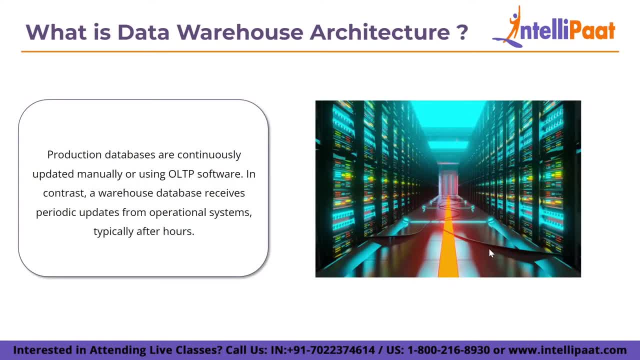 Data warehouse architecture is a very complex and complex architecture. Note that applications for data warehouses are created to support the user's ad hoc data requirements, or what's now known as online analytical processing or OLAP. Note that applications for data warehouse architecture is created to support the user's ad hoc data requirements, or what's now known as online analytical processing or OLAP. 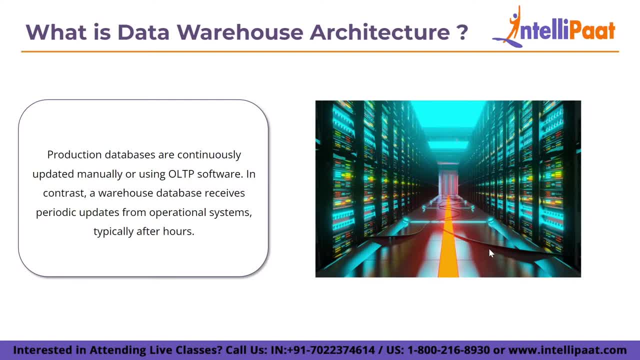 These comprise tools like trend analysis, profiling, summary reporting and forecasting. Production databases are continuously updated, manually or using OLTP software, And, in contrast, a warehouse database receives periodic updates from the operational team and is carried out multiple times every year. 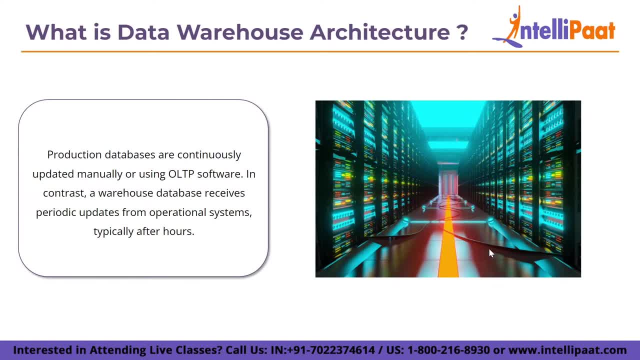 from the operational systems, typically after hours. OLTP data is routinely extracted, filtered and loaded into dedicated warehouse server that is open to user as it builds up in the production databases. Tables must be denormalized, data must be cleaned for errors and duplicacy, and new fields and keys must be added as a warehouse is filled with data. 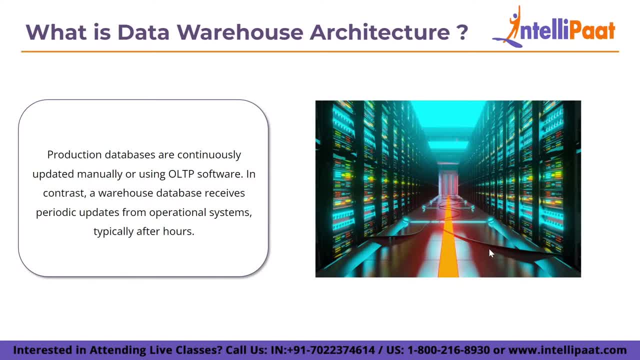 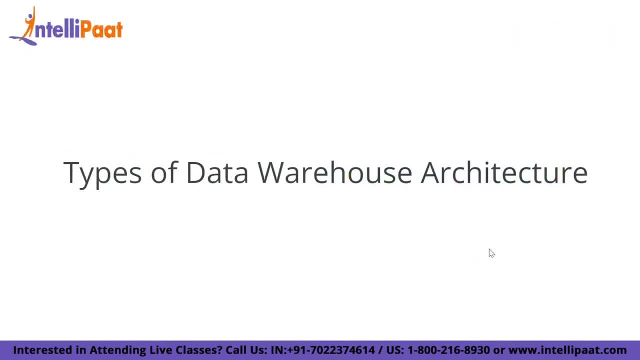 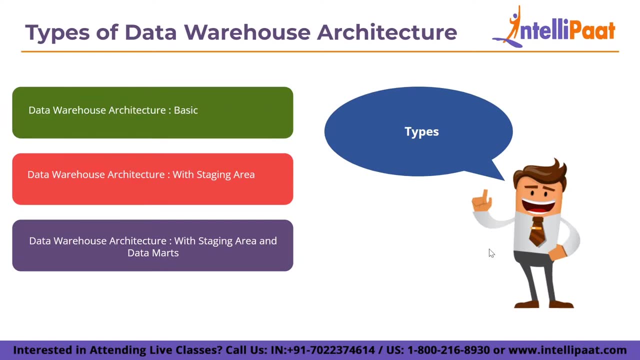 to reflect the user's need for sorting, combining and averaging data. Now let's discuss the types of data warehouse architecture. Data warehouses and their architectural designs vary depending on the circumstances surrounding an organization. The three common architectures are: data warehouse architecture basic. data warehouse architecture with staging area. data warehouse architecture with staging. 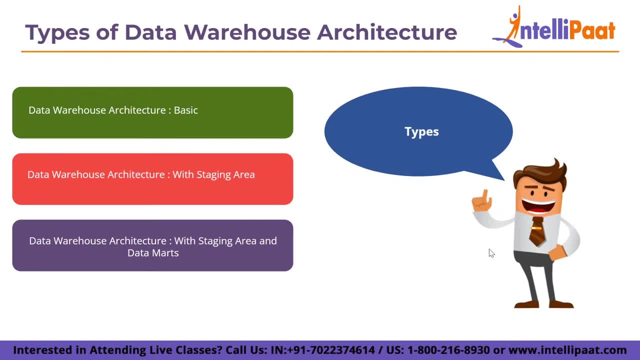 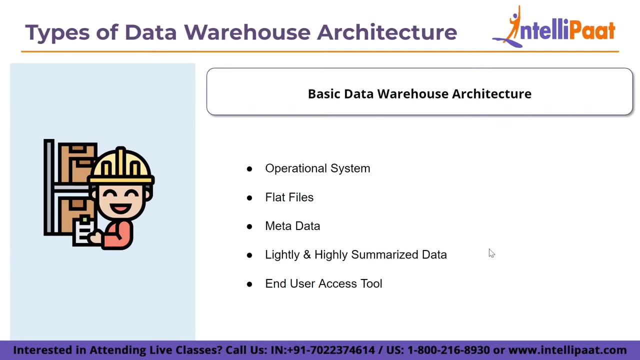 area and data marts. Now let's discuss the types of data warehouse architecture. Now let's discuss each of the architecture one by one. The first one is basic data warehouse architecture. So in this it consists of operational systems, flat files, metadata- lightly and. 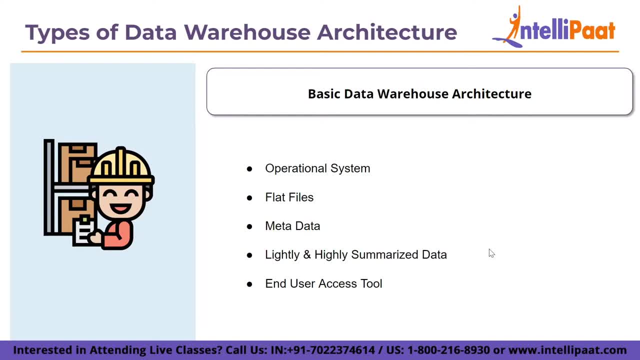 highly summarized data and end user access tool. Let's discuss one by one. If we talk about the operational system, data warehouses uses the term operational system to describe a system that handles an organization's daily transaction. Let's discuss about the flat files. Flat files is basically a group of data that describes and provides details. 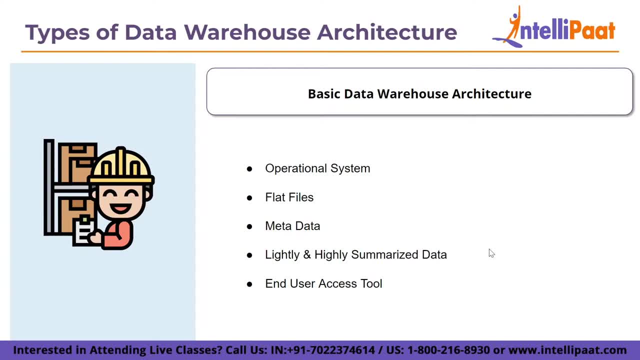 regarding other data. Every file in a flat file system must have a unique name, and it is a system of files where transactional data is stored. Now next comes is metadata. There are several uses for metadata in the data warehousing, For example, by condensing important 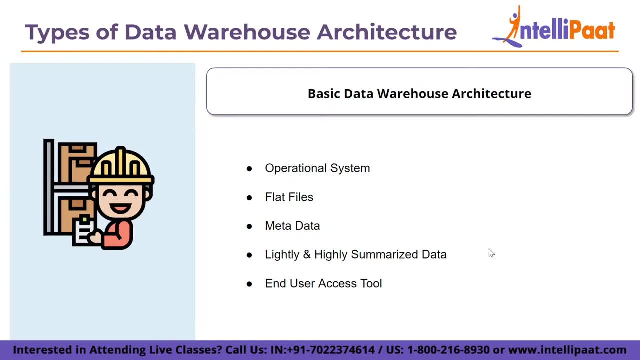 information about data metadata can make it easier to discover and use specific data instances of data. Examples of extremely simple document metadata include author data build and updated file size and data build. Now, if I talk about the next one, it is lightly and highly summarized data. All of the preset: lightweight and highly summarized. 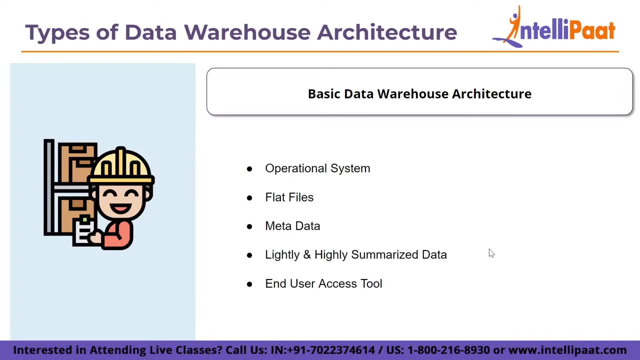 data produced by the warehouse manager is saved in this section of the data warehouse. The material has been condensed in order to improve the query performance. The consolidated record is regularly updated where fresh data is added to the warehouse And at the end we have end user access tool- A data warehouse. main objective is to give business management. 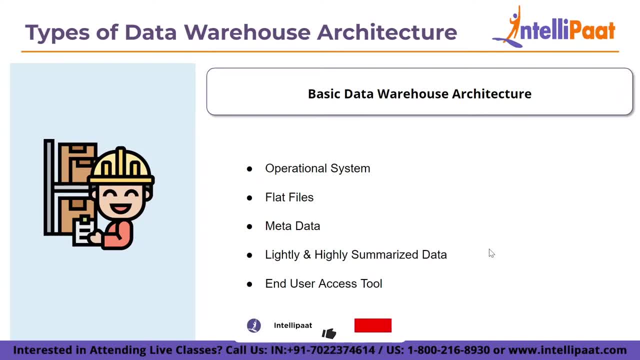 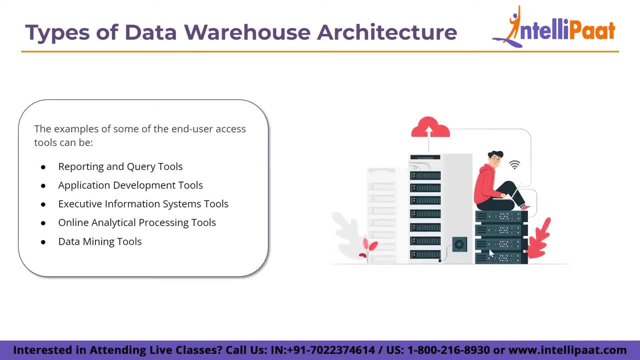 information they can utilize to make strategic decisions. These customers employ end client access tools to communicate with the warehouse. The examples of some end user access tools can be reporting and querying tool, application development tools, data warehouse and data mining tools, executive information systems tools. online analytical processing tools. 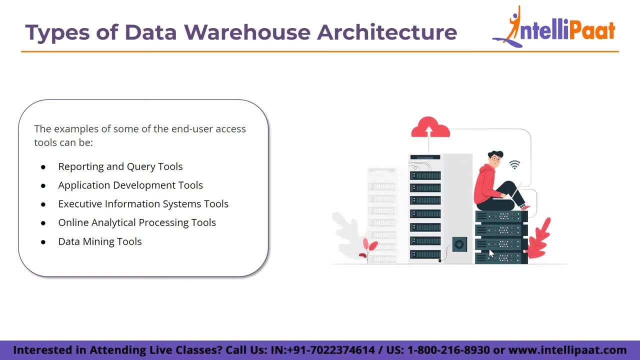 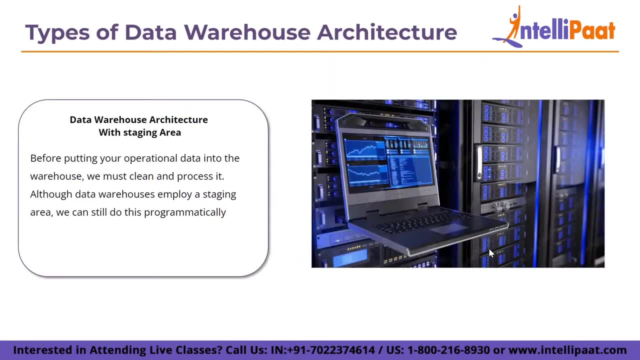 and data mining tools. So this comprises the tools for the end access users. Now let's discuss data warehouse architecture with the staging area. Before putting your operational data into the warehouse, we must clean and process it. Although data warehouses employ a staging area, we can still do this programmatically- A place where data is processed. 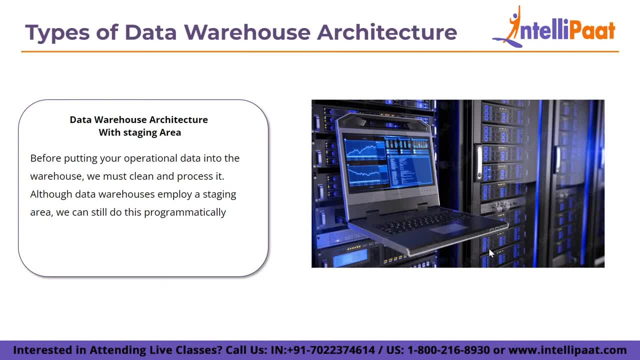 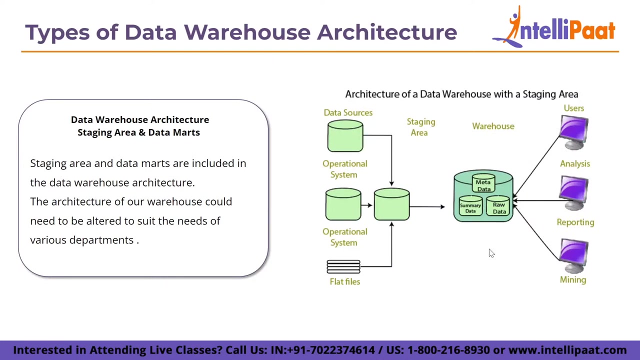 before entering the warehouse For operational methods originating from numerous source systems. a staging area makes data purification and consolidation easier, particularly for enterprise data warehouses, where all pertinent data of an organization is consolidated. Now let's discuss data warehouse architecture with staging area and data marts. Staging area. 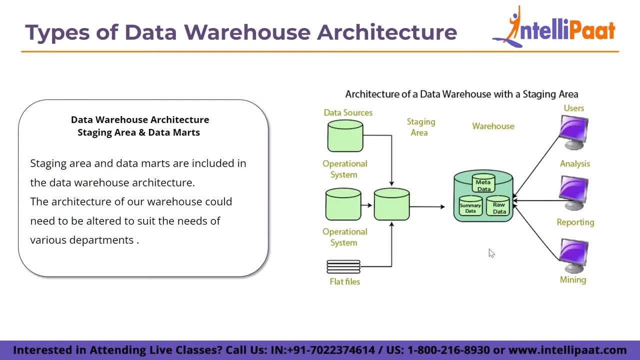 and data marts are included in the data warehouse architecture. The architecture of our warehouse could need to be altered to suit the needs of various departments. Data marts can be added to this. A data mart is a portion of data warehouse that can give data for reporting and analysis on a division, unit, department or activity. 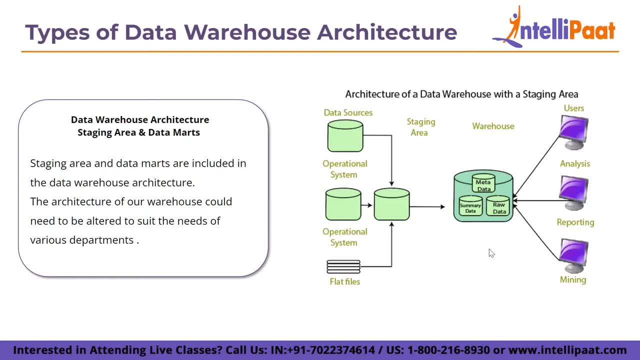 within the business, such as sales, payroll, production and etc. The figure shows here a scenario where stocks, sales and purchases are handled separately. In this illustration, a financial analyst wishes to examine the previous data on sales and purchase or mine historical data to forecast the consumer behavior. 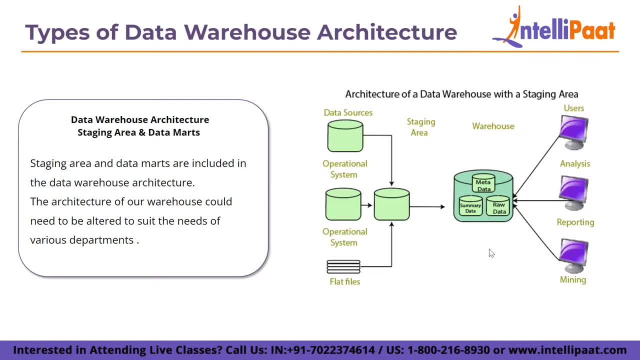 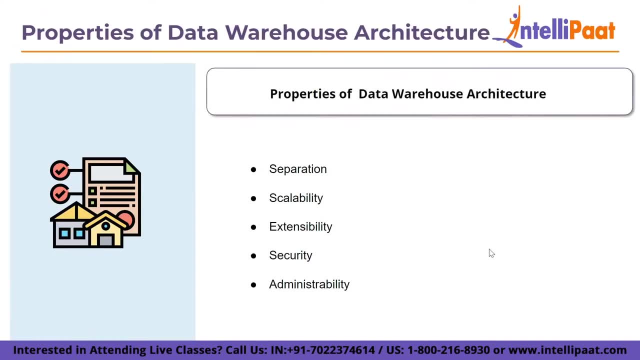 So this was the data warehouse architecture, with staging area and data marts. Now let's discuss the properties of data warehouse architecture. The first one is separation. It is best to keep analytical and transactional operations separate as much as feasible. The second thing comes as scalability. Scalability means that 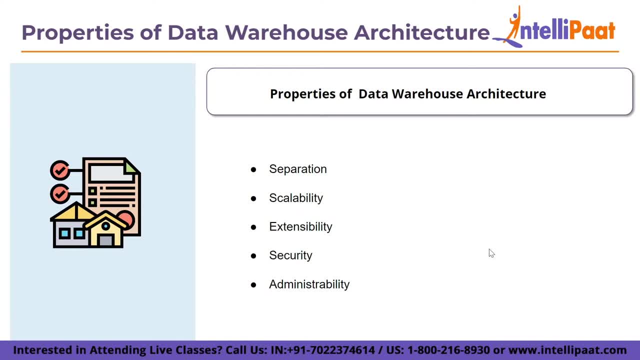 the data warehouse is separated from the data warehouse. The second thing comes as scalability. The third thing comes as scalability. The fourth thing comes as scalability. The fifth thing comes as scalability. Hardware and software architectures should be easy to upgrade as user requirements and the amount of data that must be managed and processed grows along. 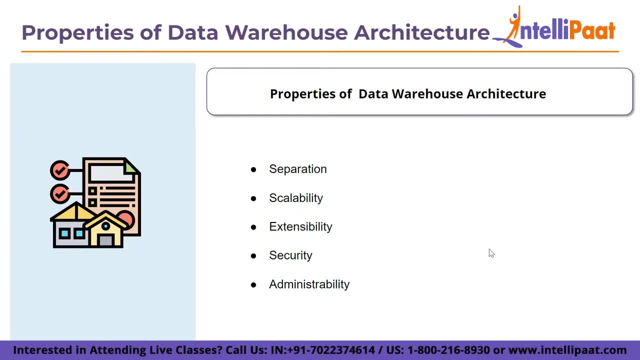 with the numbers of users. The third thing is extensibility. The architecture must be adaptable to new functions and technological advancements without requiring a complete system overhaul. Fourth one is security. If I talk about the security due to the strategic data kept in the data warehouse, accesses must be monitored. And the final is administrability, Which means 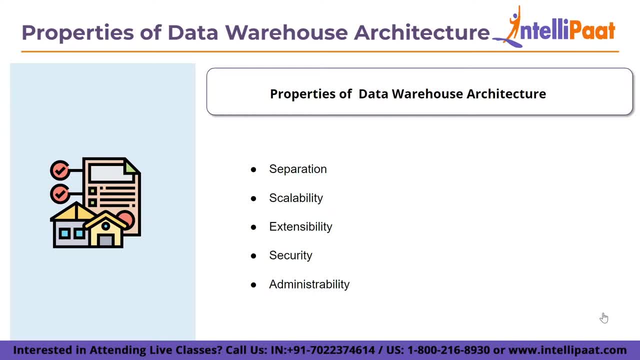 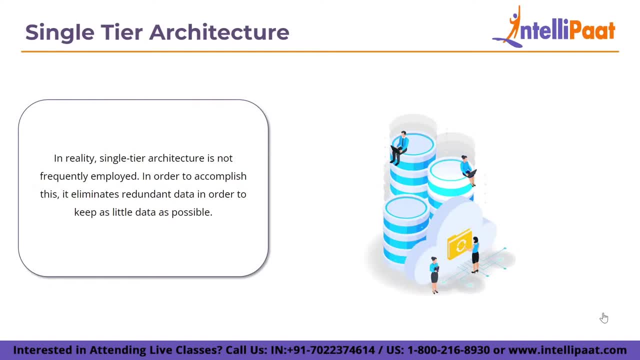 that managing a data warehouse shouldn't be at all difficult. Now let's discuss the single tier architecture. So, in reality, single tier architecture is not frequently employed. In order to accomplish this, it eliminates redundant data in order to keep as little data as possible. The source: 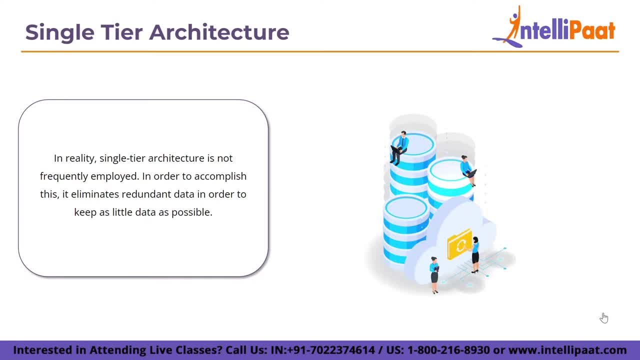 layer is the only layer that can be used to manage the data warehouse, So, in order to layer that is actually accessible, It demonstrates that data warehouses are virtual in this approach. This indicates that data warehouse is actually a multi-dimensional representation of operational data produced by the particular middleware or intermediate processing layer. 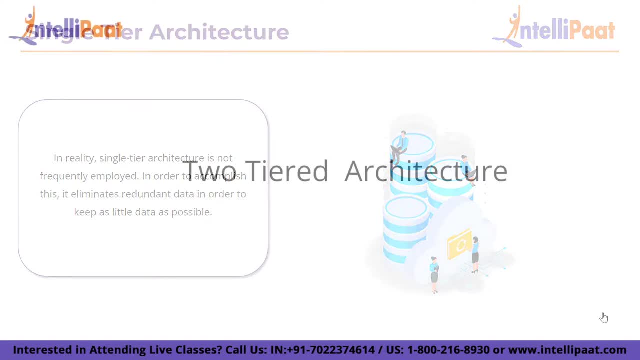 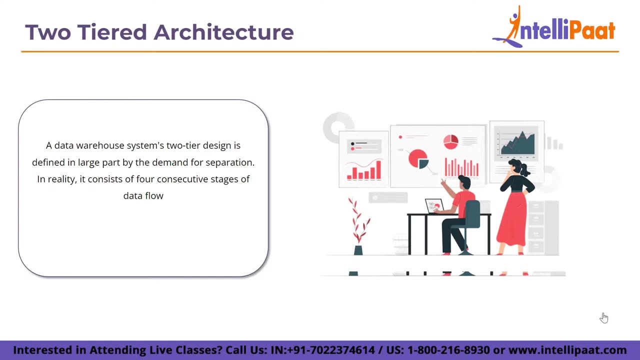 Now we gonna go through the two-tiered architecture. A data warehouse systems is a two-tiered design which is kind of defined in a large part by the demand for separation, Although it is frequently referred to as two-layer architecture to emphasize a division between physically accessible sources and the data warehouses. 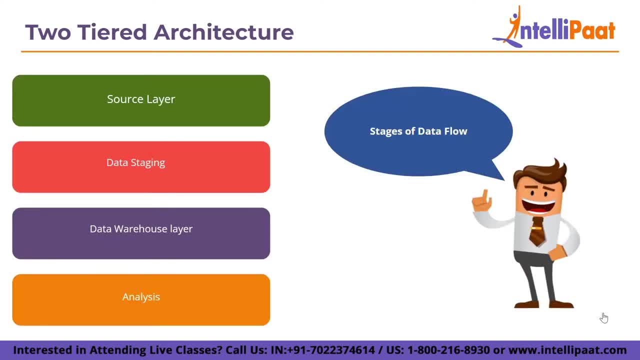 But in reality it consists of four consecutive stages of data flow. The first one is source layer. If I talk about the source layer, data warehouse systems use variety of data sources as their source layer. The information may originate from an information system beyond the data warehouse. 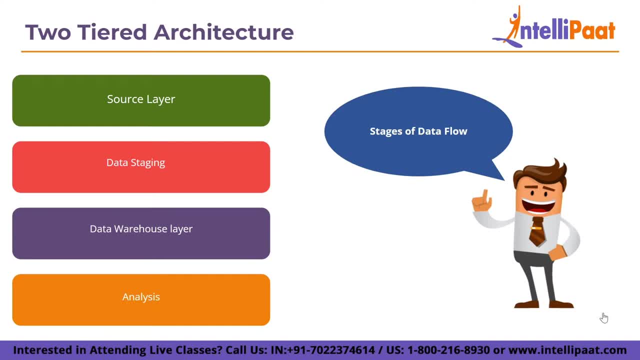 The second is data staging. Data staging entails extracting the data from the source, cleaning it to remove discrepancies and fill in any gaps, and integrate it to combine data from several sources into single-stranded schema. The so-called extraction, transformation and loading tools may extract, transform and clean. 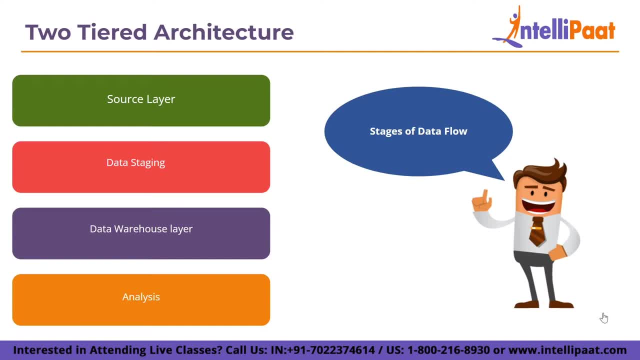 data validate, filter and load source data into the data warehouse, while combining the disparate schemata Now the third one is data warehouse layer. A data warehouse serves as a logically centralized one-store for information. The data warehouse can be accessed directly, but they can be also. 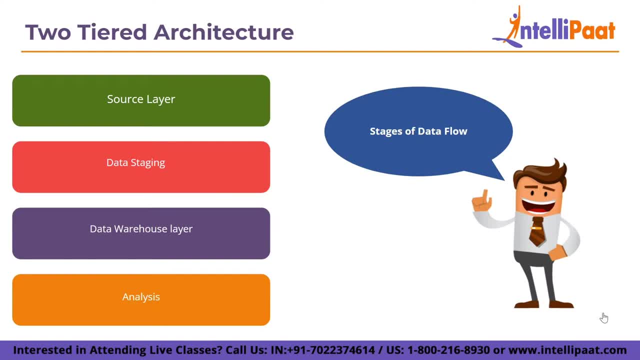 utilized as a source for developing data marts, which are intended for particular company departments and partially reproduce the contents of data warehouses. Data staging, users, sources, access processes, data mart, schema and other information are all stored in the metadata repositories, And the final one is analysis. If I talk about this layer, it allows for rapid and flexible. 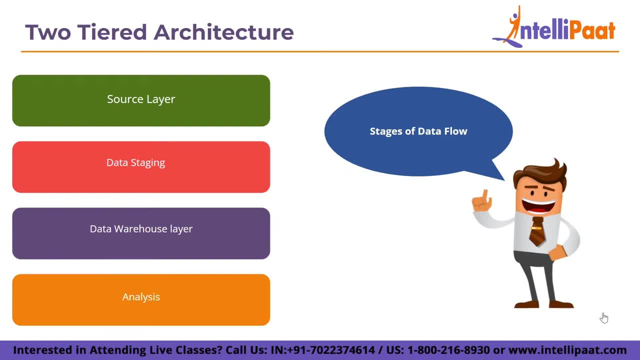 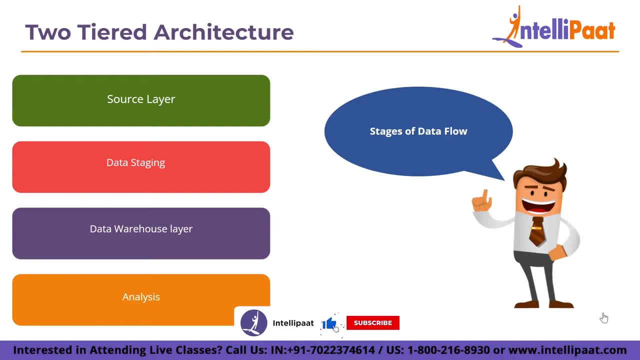 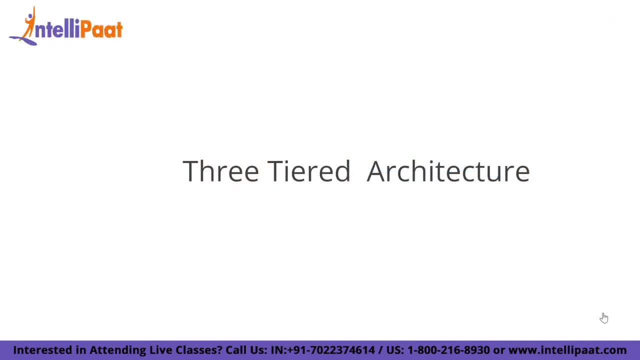 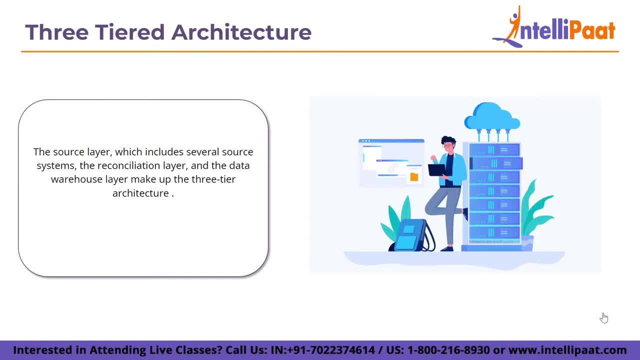 The source layer in the three-tiered architecture includes several source systems. The reconcilation layer and the data warehouse layer makes up the three-tier architecture containing both data warehouses and data marts, And between the data warehouses, the source data is the reconciliation layer. 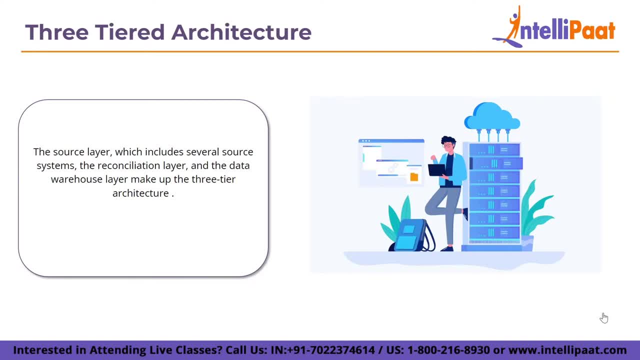 The reconciliation layer contains the data warehouses and the data. marts layer's key benefit is that it produces a uniform reference data model for the entire company. It also distinguishes between issues with data warehouse fillings and those with source data extraction and also integration. In some instances, the reconciled layer is also used directly to 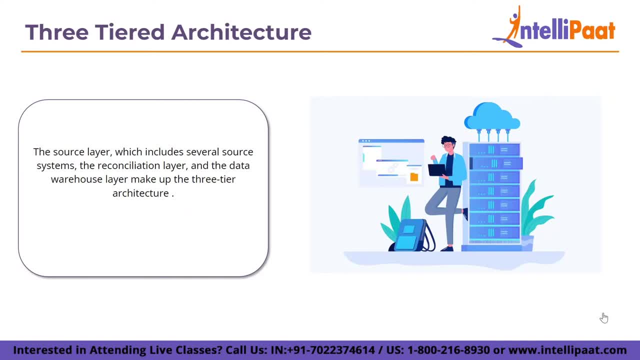 improve how some operational tasks are carried out, such as generating daily reports that cannot be adequately prepared, using corporate applications, or creating data flows to periodically fill external processes in order to gain the benefits of cleaning and integration. Particularly beneficial for the large enterprise-wide systems, this architecture is 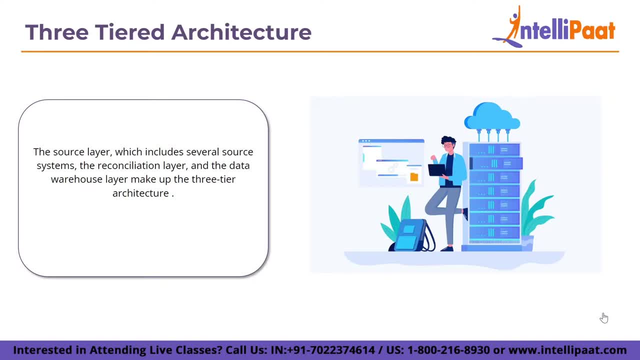 particularly beneficial for large enterprise-wide systems. The additional file storage space required by the extra redundant reconciling layer is a drawback of this arrangement. The analytical tools are also little less Real-time as a result. the typical three-layer architecture of the data warehouse consists of: 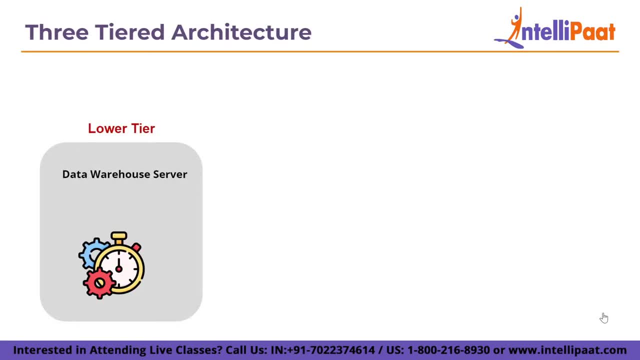 the following: The first one is the lower tier, or the data warehouse server. The second one is the upper tier, or the OLAP server, And the final one is kind of top-notch, or the front-end tools. An RDBMS-based data warehouse server makes up the bottom tier of this architecture. 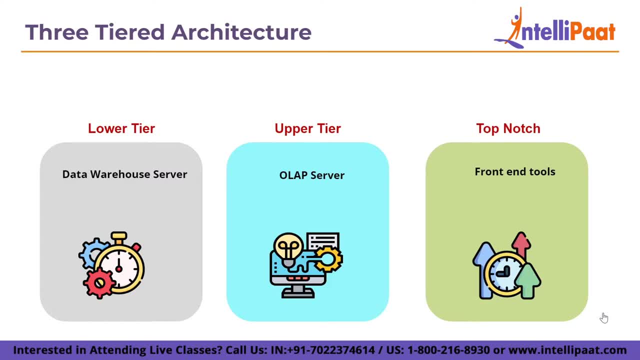 It might contain a metadata repository and a number of specialized data marts. Using application program interfaces known as gateway, data is pulled from the operational databases and external sources, such as user profile data provided by the external consultants. The underlying DBMS provides a gateway that enables client programs to create SQL code. 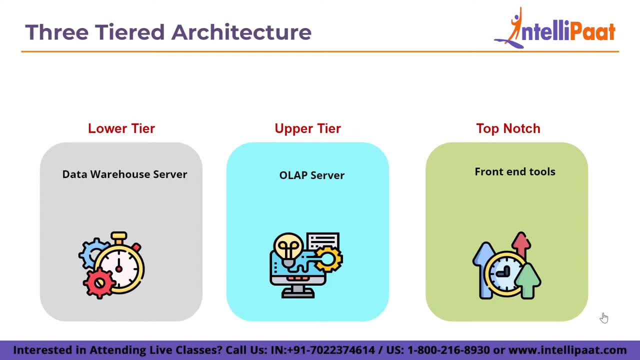 for the server execution. If I talk about a middle tier, that includes the OLAP server for quick data warehouse queries. In order to implement the OLAP server, we have the first one, a RDBMS-based data warehouse server, a relational OLAP model, which is often known as the extended relational database. 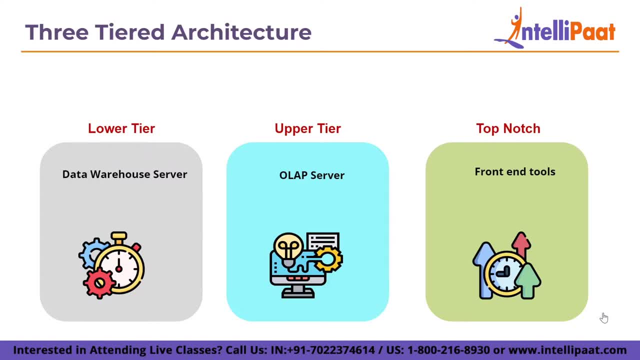 management system, which converts multidimensional data functions into common relational operation, And the second one is multidimensional OLAP or M-OLAP. This model, which is a special purpose server that carries out multidimensional operations and information directly. It includes a tool for data mining for the OLAP generated data, as well as front-end tools for showing. 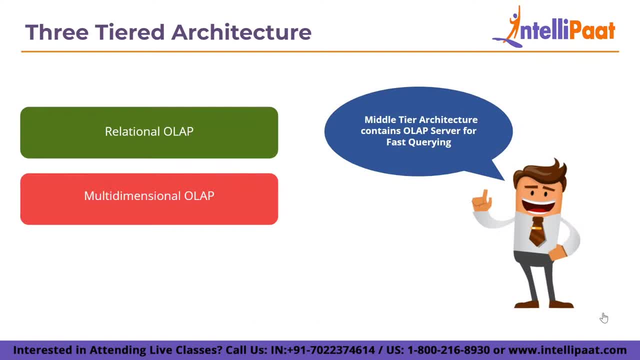 findings from the OLAP. So in the three-tiered architecture we have relational OLAP and the multidimensional OLAP. for the middle tier architecture It also contains OLAP server for the fast querying. Now let's discuss the principles of data warehousing. 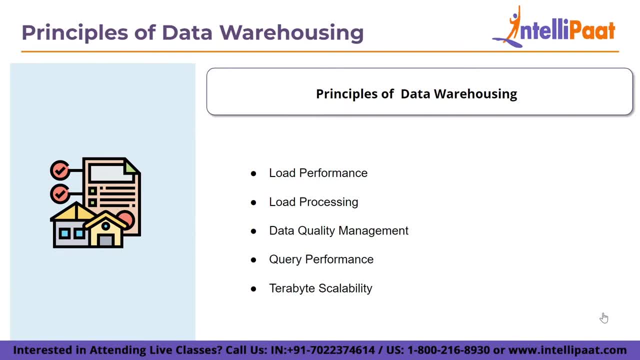 These are the following principles of the data warehousing. The first one is load performance. Data warehouses need to continuously load more data on the regular basis within constrained time periods. The performance of the load process should be measured in gigabytes per hour and hundreds of millions of rows, without arbitrary limiting. 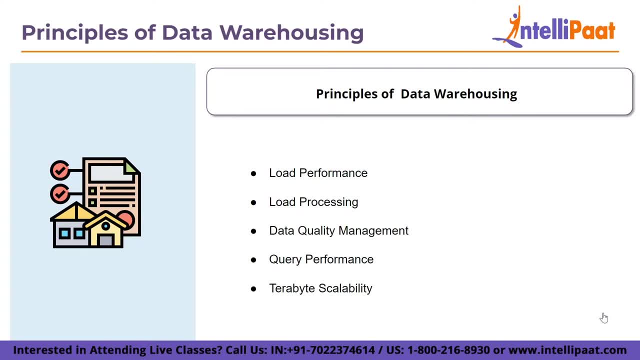 the amount of data that can be processed. Next one is load processing. Data conversion, filtering, reformatting, indexing and metadata updating are just few of the many steps that must be completed before adding new or updated data to the data warehouse. The third one is the data quality control. The utmost data quality is required for the